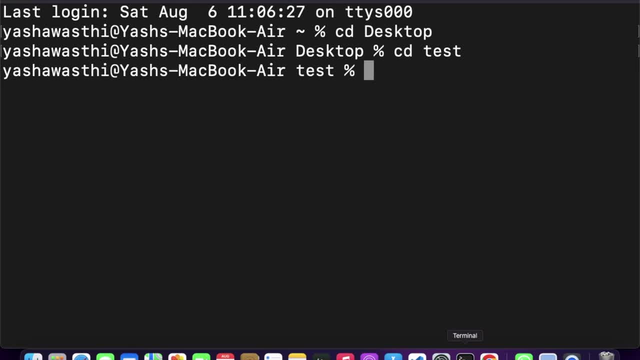 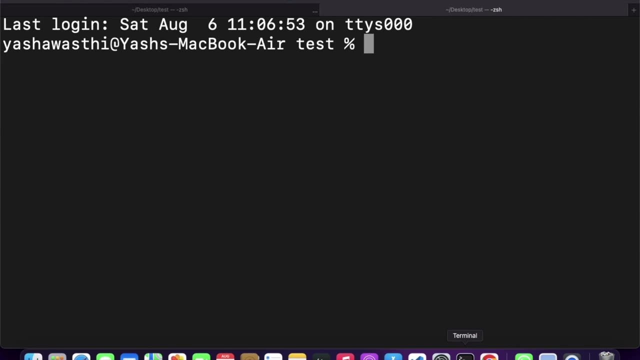 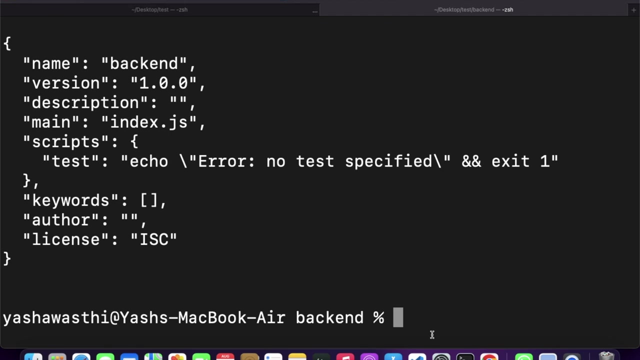 will change directly to test. Now we will say make directory and we will say frontend and backend and we will switch tab and we will say change directory to backend and here we will say touch index, dot, js. And now we will say npm init, yes, and we will hit enter. Now we can say that npm install. 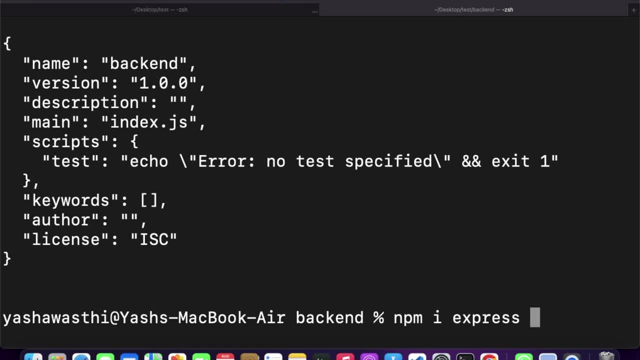 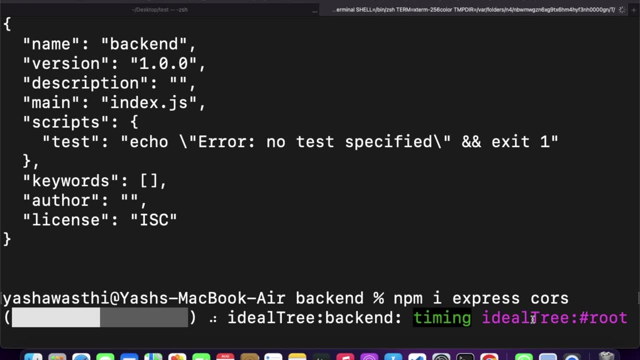 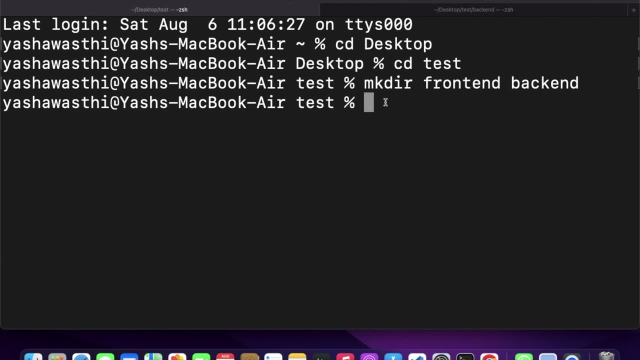 express, which is a package we will need, and we will say course as well and we will hit enter, So this will install express and course into our backend. and now we will go to our frontend and we will say: change directory. So frontend, npx, create react app dot slash. So this will create our react app and while 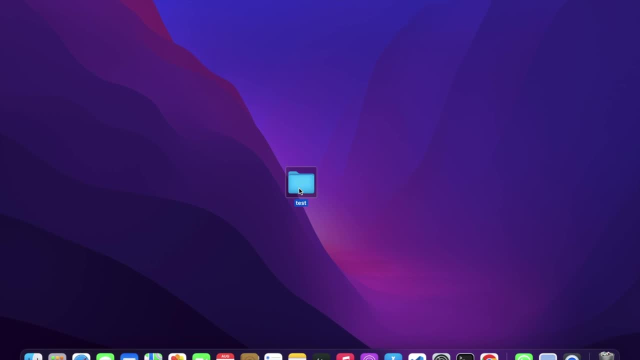 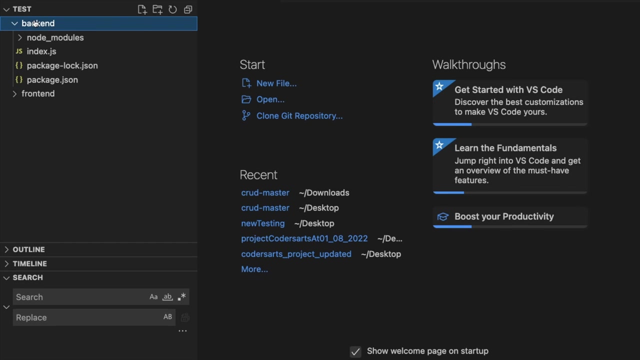 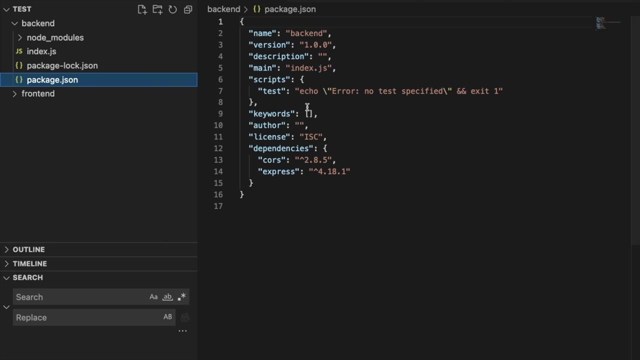 it is creating it. we will drag this folder into our vs code. We will drag it here and while going into backend To do one thing, we will go to our packagejson and beside this main we will hit enter and say type module. So this would help us use import and we will not be required to use require keyword. so 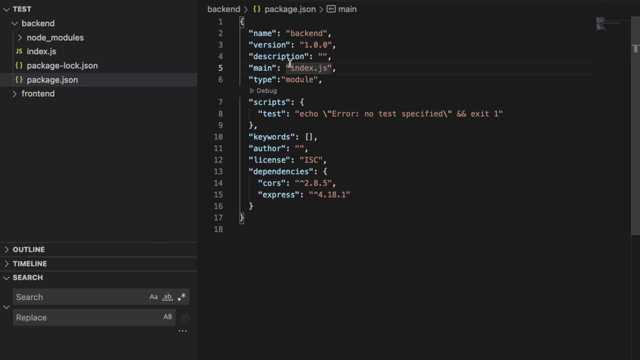 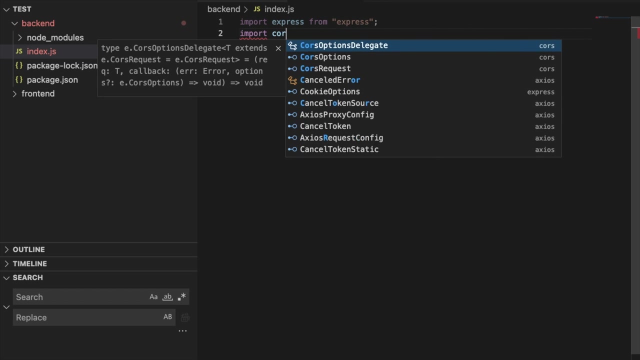 this would help us And now we will save. We will go to indexjs and we will start by writing import express from express. Then we will say import course from course, And then we will say importjson from course, And then we will say: const app is equal to express. 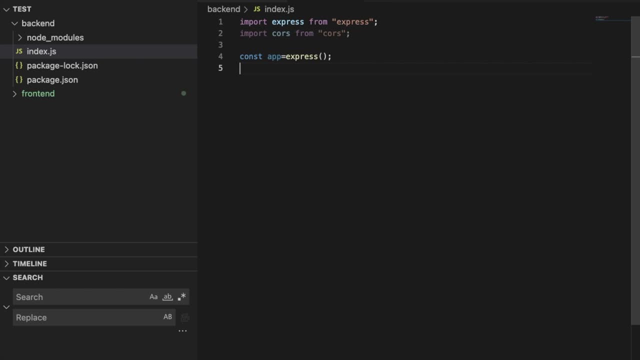 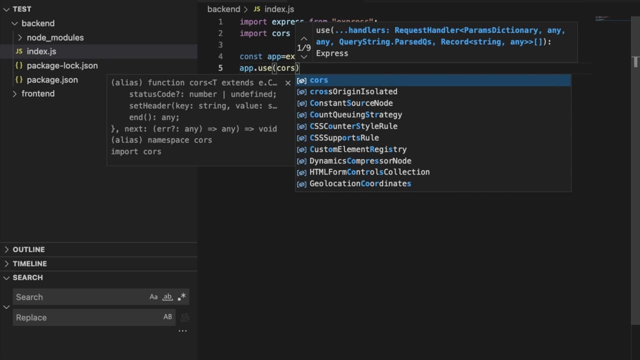 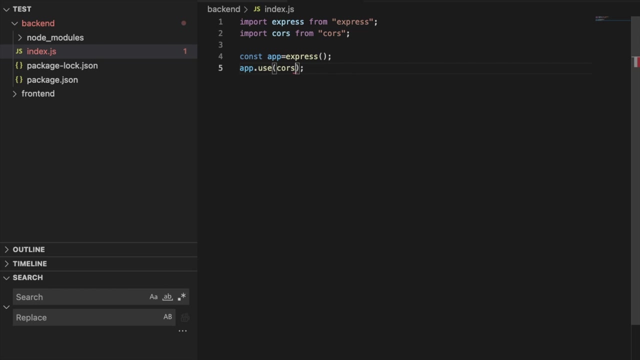 So this would create our app, and then we will say: app dot use course, right, I think we have placed a lot of brackets there. and then we will hit enter again and then we will say: Now, this is what we have done. We will say: app dot listen to, app dot listen. 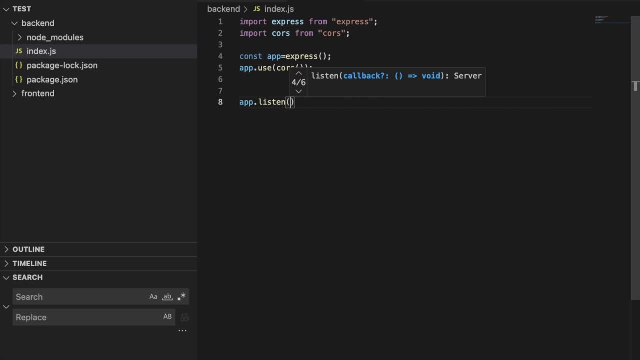 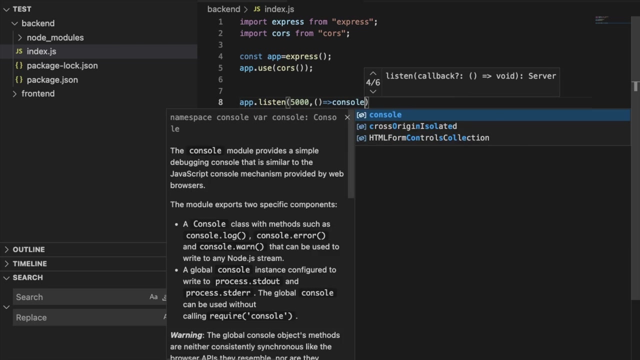 To port 5000. this is the port we will be listening to and we will say when we start listening, we will say: console dot log app is running Now, we are going to run it, We are going to run it, We are going to run it. 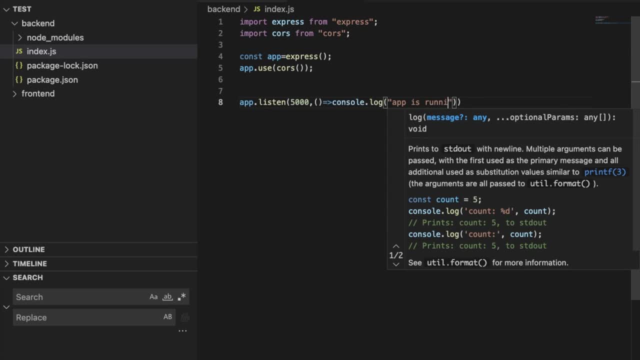 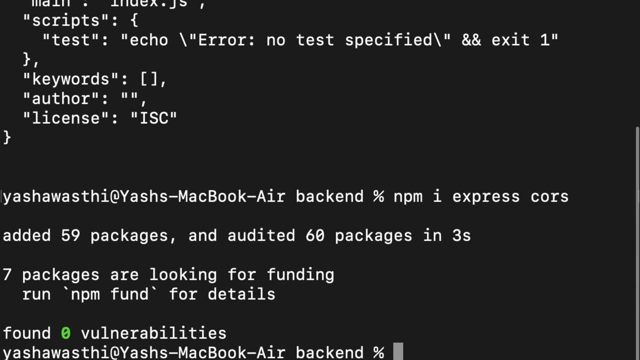 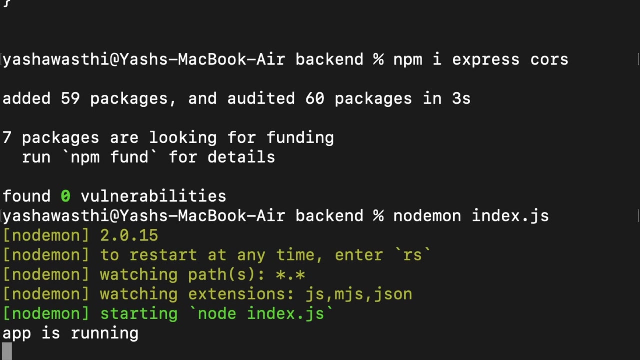 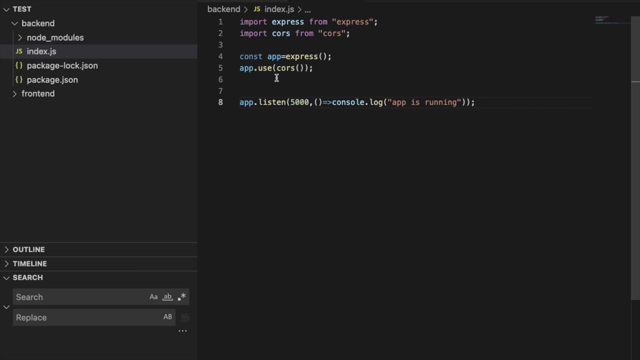 Now we are going to run it. We are going to run it running, we will save this and we will go to our back end and we will say: nodemon indexjs. this would start our back end and you can see app is running now. first we will test that our back end is sending the data to our front end, or 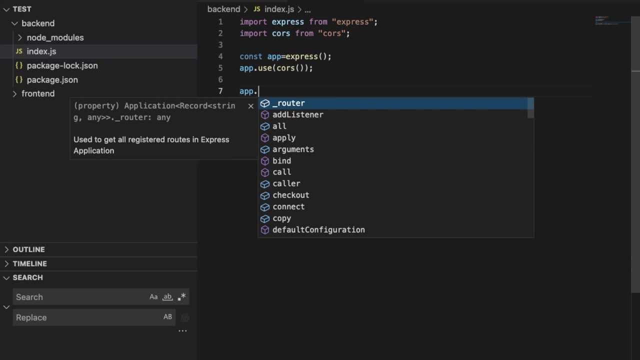 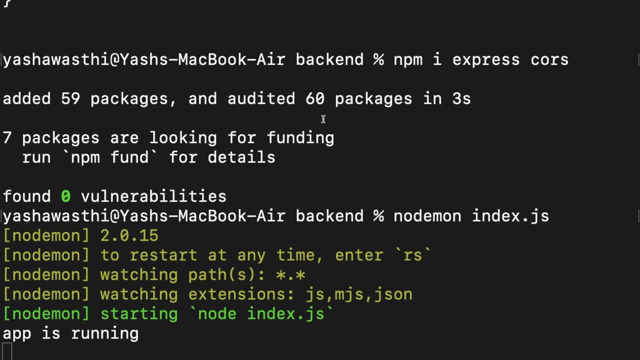 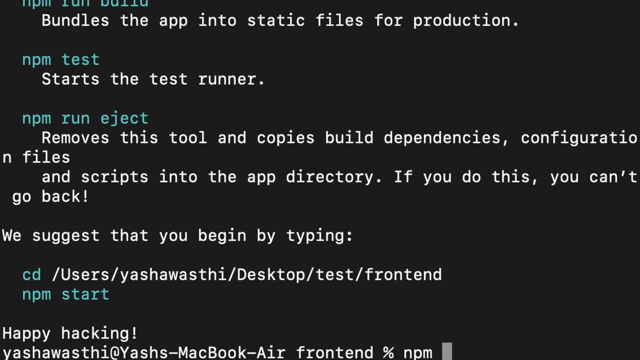 not. so for that we will say appget, and we will say: okay, we can. uh, the one thing we can, just directly, we can call that in our back end, in our front end, and then we can test that. so in front end we can say: m start, this would start our development server. 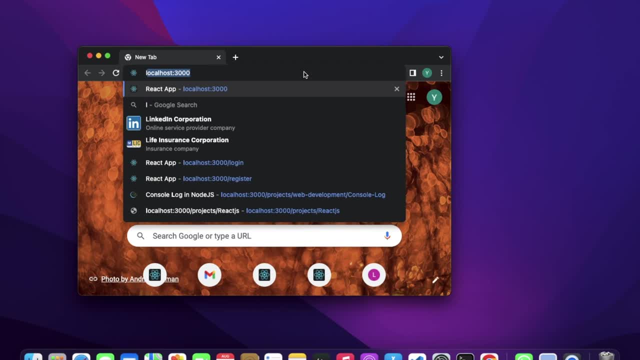 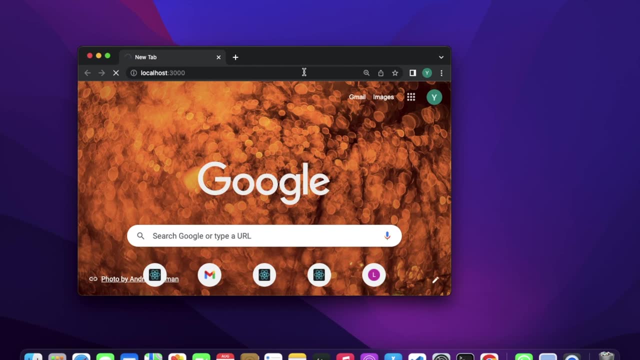 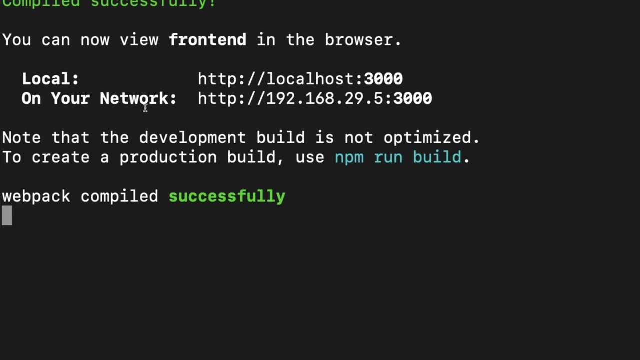 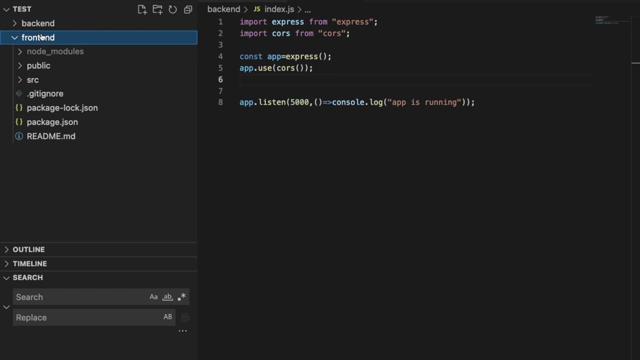 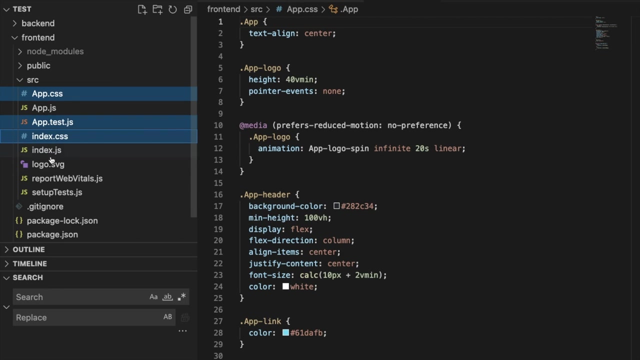 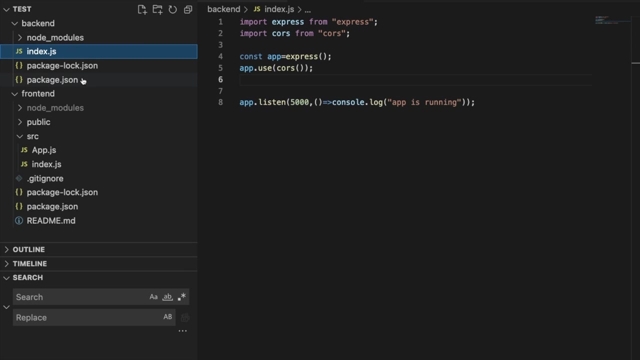 so our development server is running, also running. so we will do one thing: we will close this for a moment and we will go to source. we will delete all these files which we do not need. our goal here is to just check how we can send and receive data, so we will not be concerned. 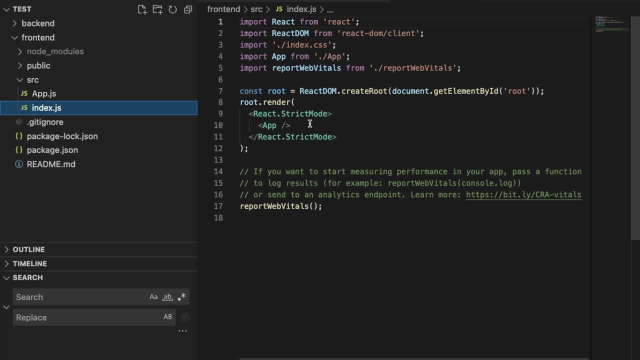 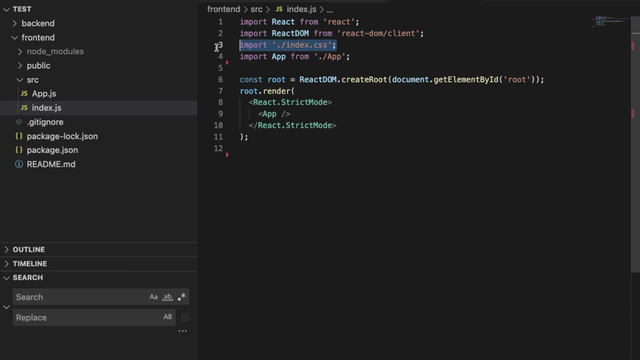 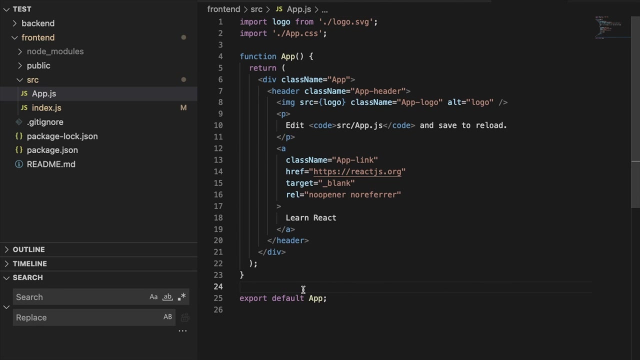 about the styling. so we will go to index and we will delete this. we will delete this as well and we will delete this and we will hit save and in appjs we will completely remove all the things and we will use this snippet to create app and we will hit save so we can see that our app shows here now. 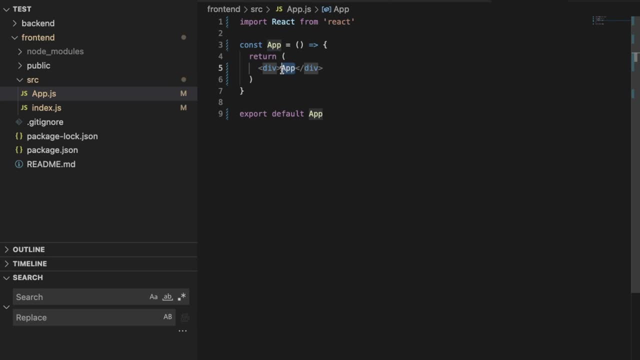 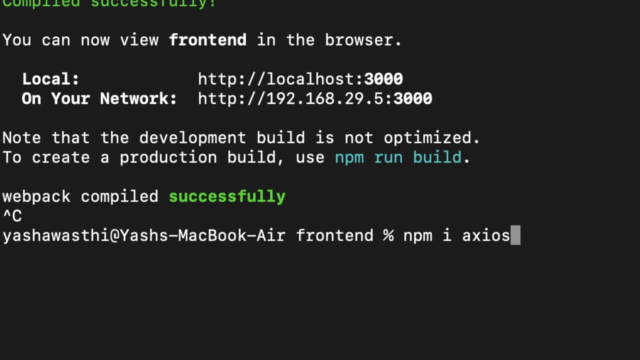 you. I want that this app, this text app, should not show this particular hard coded app, but something which we will receive from backend. so for that we'll have to use axios. so we will first of all go to our terminal and we will say: npm, install axios and we will hit enter. 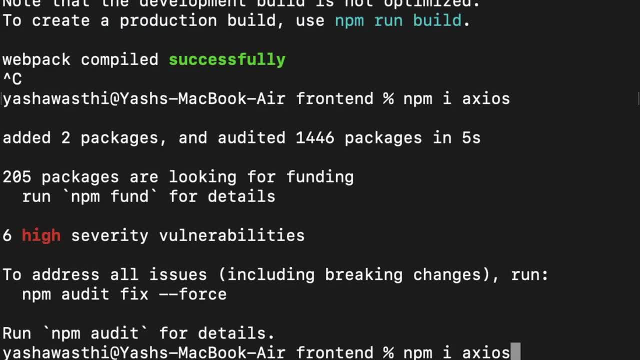 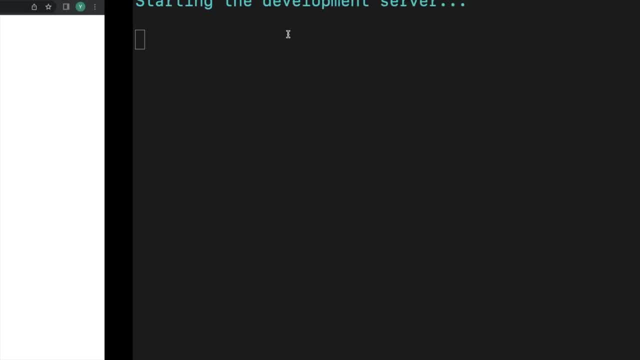 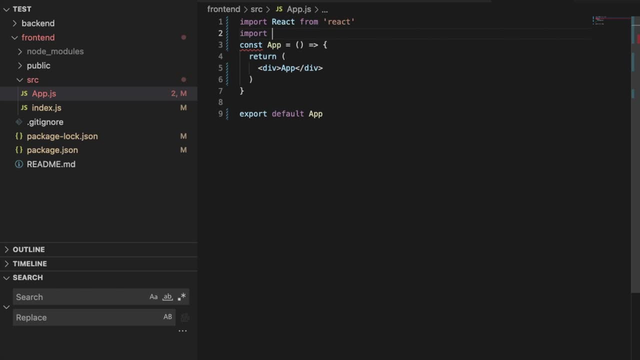 okay, so axios is installed and you can say: npm, start now. and here. so you can say: import axios from axios. so axios is used to send and receive requests to the backend. so now we will go here and we will say const data, set data. data is equal to use state and we will hit enter. so this we can use to get the data which. 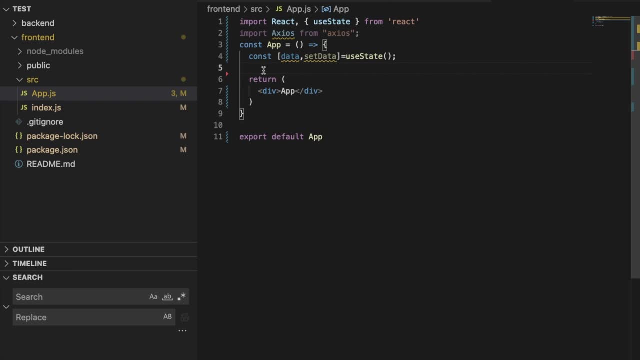 we receive from the backend, and here we will say, once get data is equal to a sync function and we will say thorns response is equal to await axios dot get, and we will say HTTP localhost 5000, because it is the port which we are listening at, and we will say data or get data. 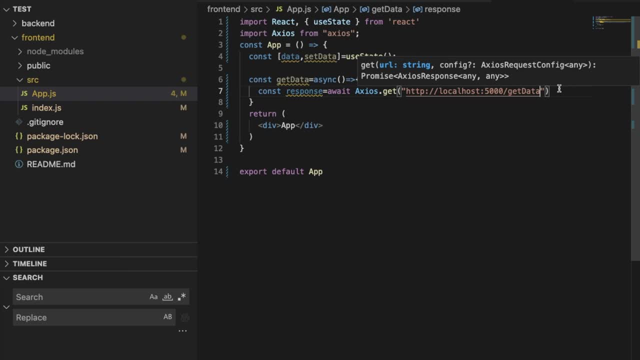 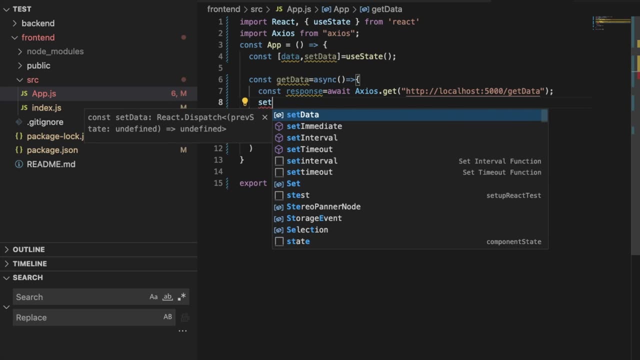 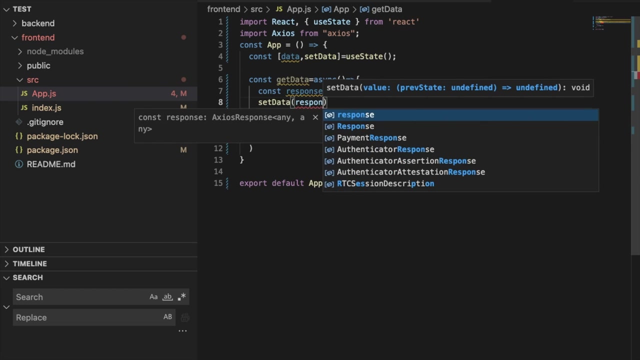 right, so this we have done. and as soon as we leave this, so we will say: set data which is this one moves this form, tell us the data right. and here we can specify that this is a text or strent, and here we will say: we will show data here. right, we will show data here. and by going here, 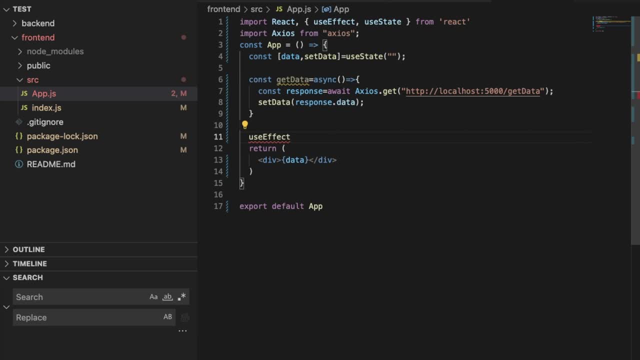 we'll say use effect and we will say get data, which is this function. they will call that as soon as the player page loads and specify it right. So our front-end is built now. as for behind, we are hide the text, if basically ready. we have specified axios imported, we have made up data and we can. 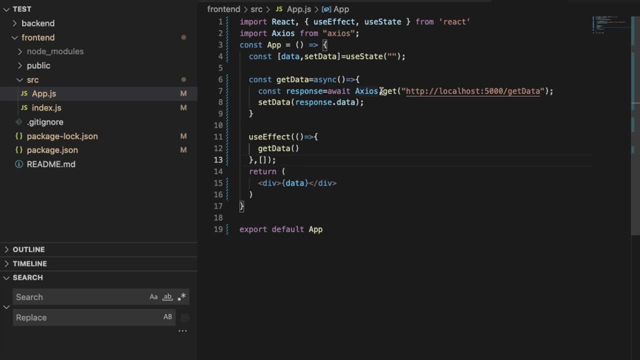 we have all. we have requested the data from back-end using axios on the port 5000 and get data, and we have used use effect and the data which we see which will be that will be shown here. so these are the things which we have done till. 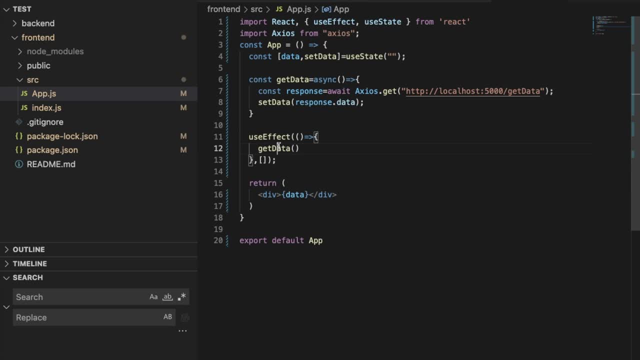 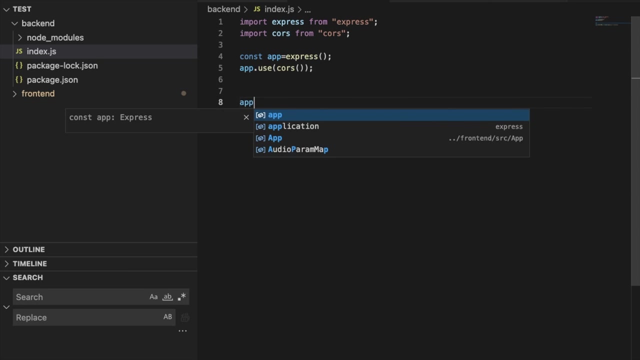 now. now we will save this. as you can see, this would not show anything because data is currently empty. so we will go to back end in indexjs and we will write when appget as our request which we are sending here. you can see that it is a get request, so we can say appget and when we 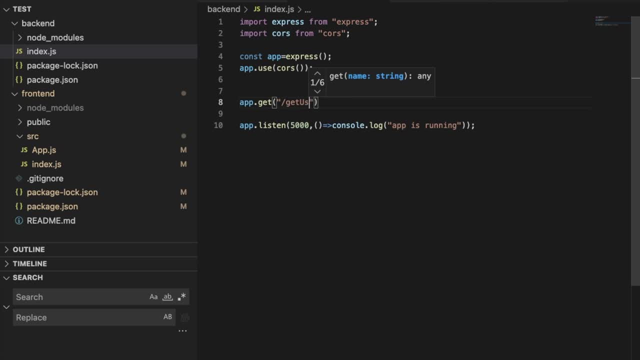 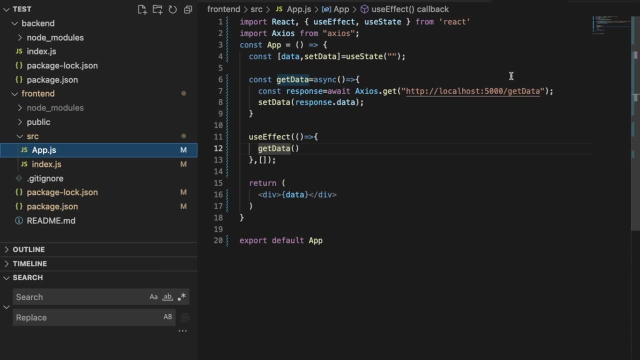 say that it is a get request, so we can say appget. and when we say that it is a get request, so we can say appget. and when we receive a get request saying get users, I'm sorry, I'm sorry, get data is the word I specified. yes, you can copy that so that, because this would create error if 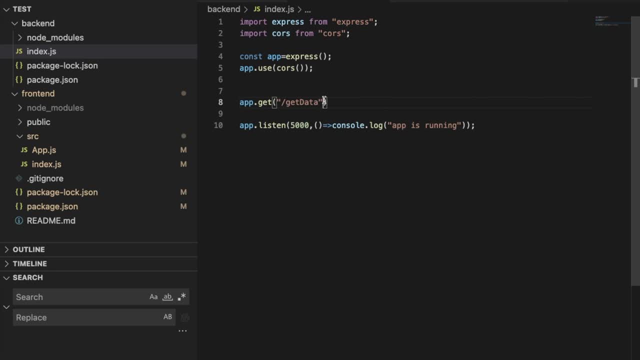 we, although the same, but it is a good practice to copy that and we will say that if this, we get this specified text as a get request, so we will say let's press press, which is short form for that question response, and we will specify that response dot send. 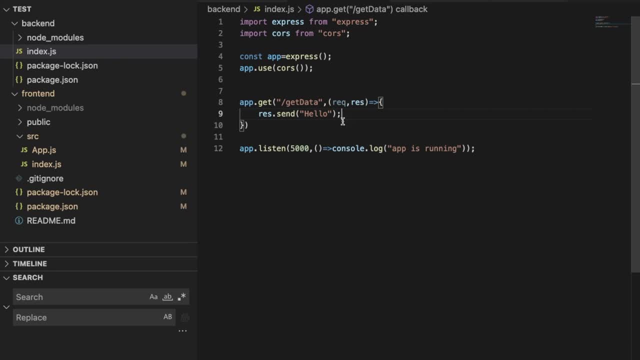 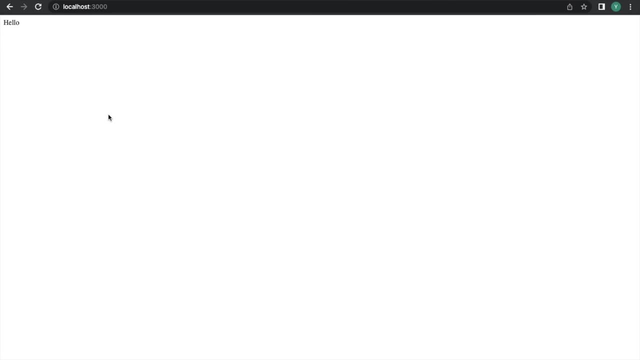 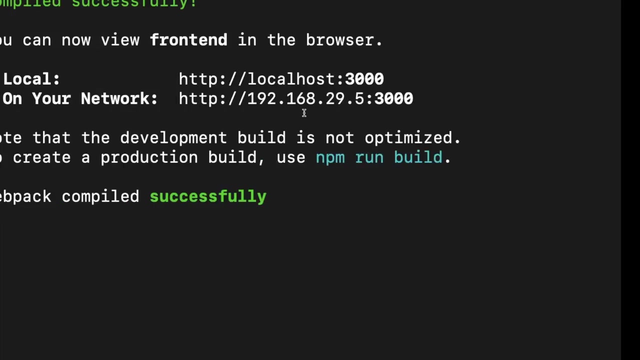 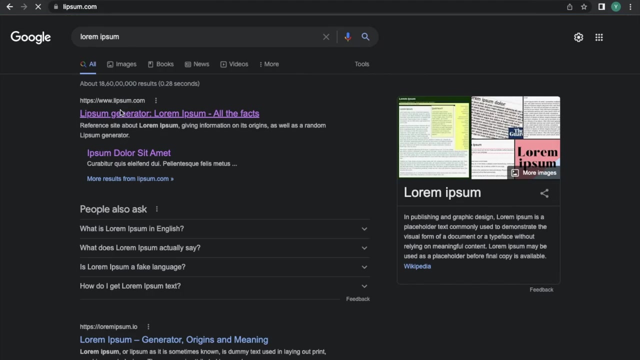 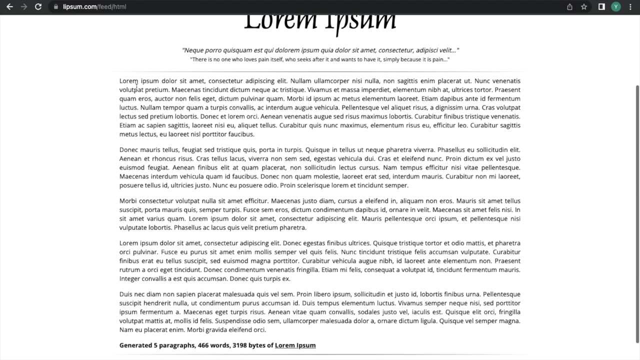 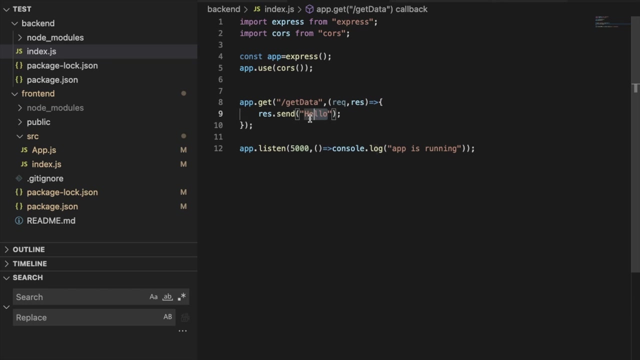 hello and we can save and you can see this hello appears here, so I could have written like you can go to lorem ipsum, you can generate a text of five paras maybe, and you can copy that and I could have sent this entire text here. okay, because that changed lines. that is why it is saying this cause. 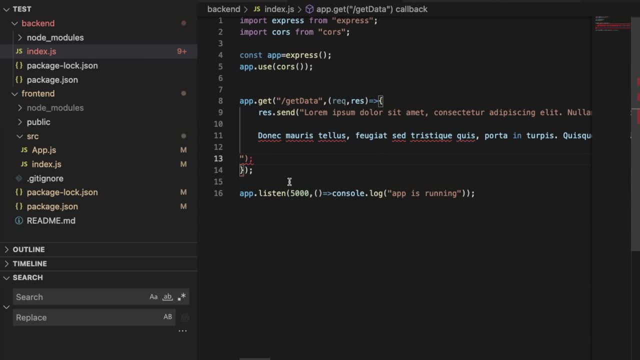 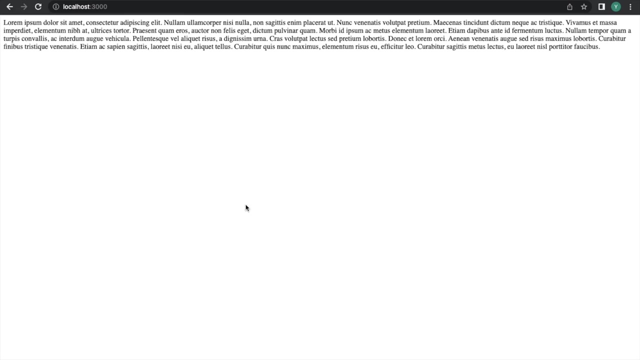 error, so we can delete this. you can delete it, don't need this. one line would be sufficient and we will say: right, huge text. and we can see that if we reload the complete text we received in our front end. so this is the result of that which we can see. of course, we can delete it, which means that one line will be.